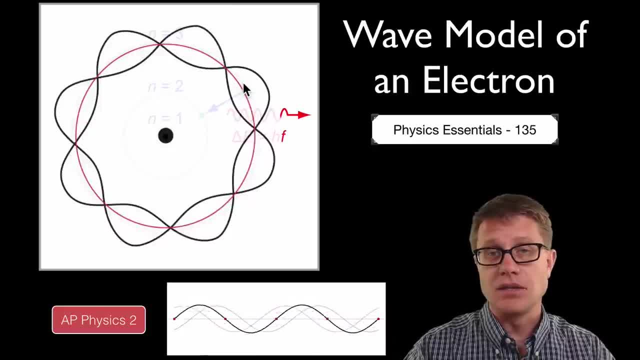 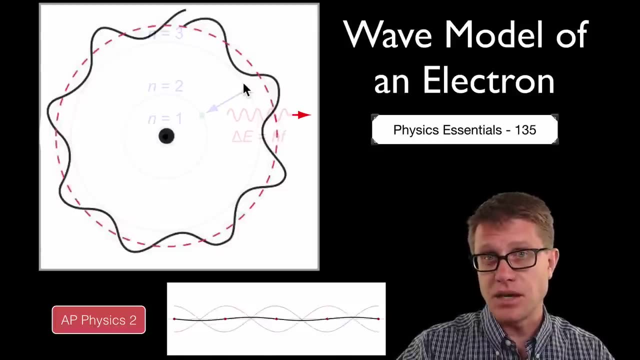 around the outside of the atom is interfering with the electron itself, And so what you get are these standing waves that build up, And that is where that energy allows the electron to be there. But in between these different orbits they do not match up perfectly, And so they have to be a whole integer of the wavelength. 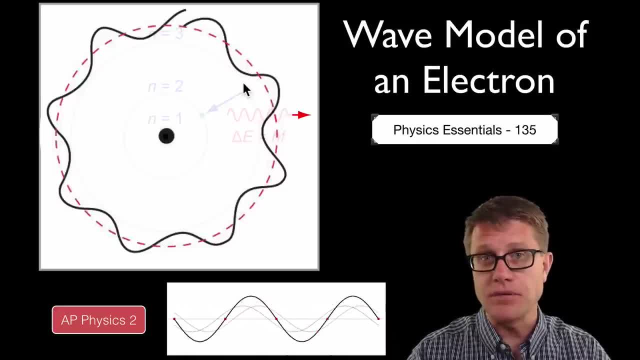 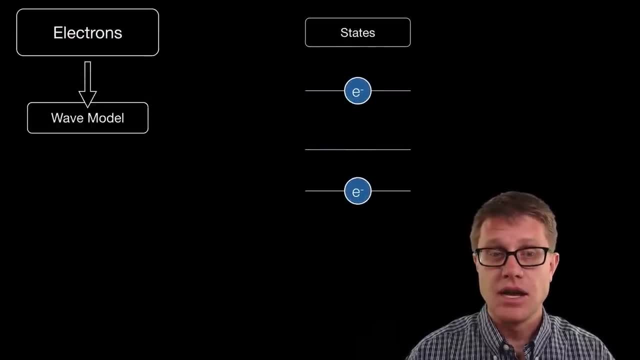 the de Broglie wavelength for the electron to exist. If it does not match up perfectly, then the electron annihilates itself, And so electrons can only exist in certain energy states, And so the wave model allows us to understand this at the level of standing waves. 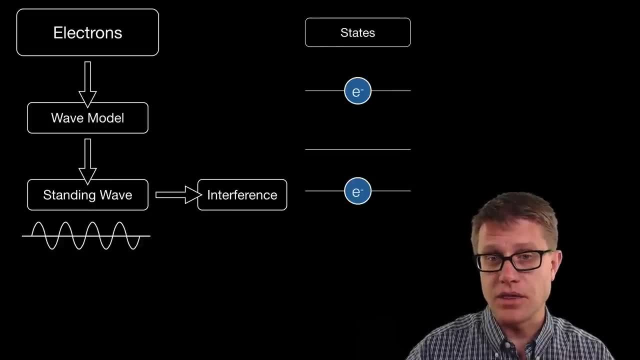 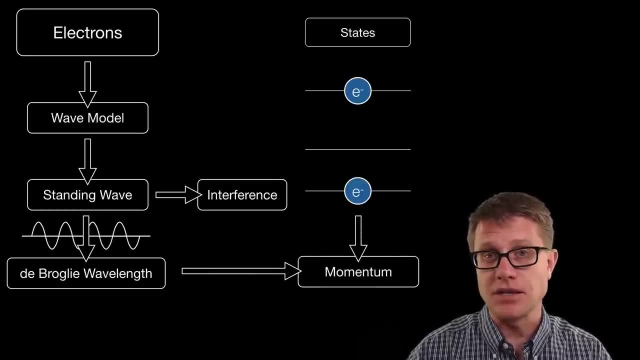 And so standing waves occur when the waves are interfering with themselves, And so the de Broglie wavelength showed us what that wavelength is, And then we could use that to calculate the momentum and even figure out what is the size of the atom itself. Another: 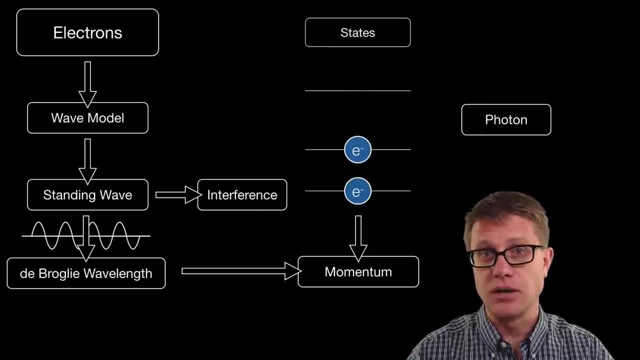 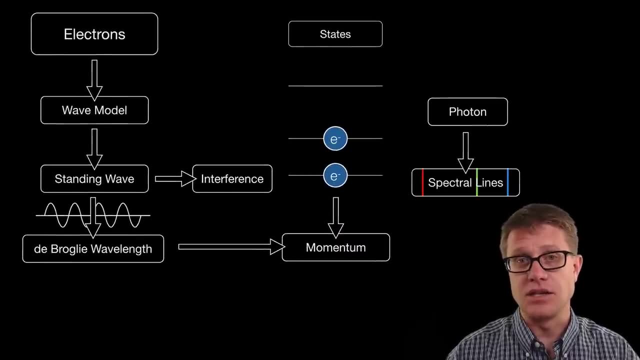 important thing it showed us is that, as electrons fall to a lower energy level, that energy contained within that standing wave is released, and released in the form of a photon that we can see in these spectral lines. So to really understand what is going on with these, 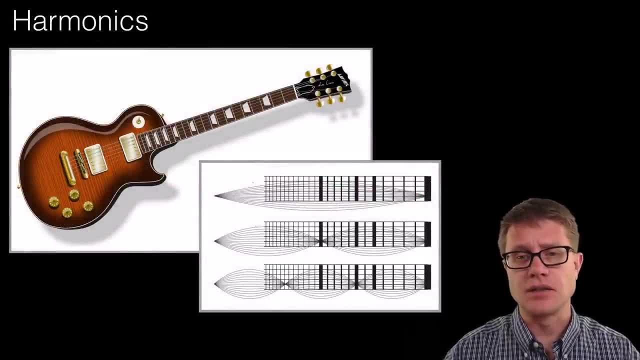 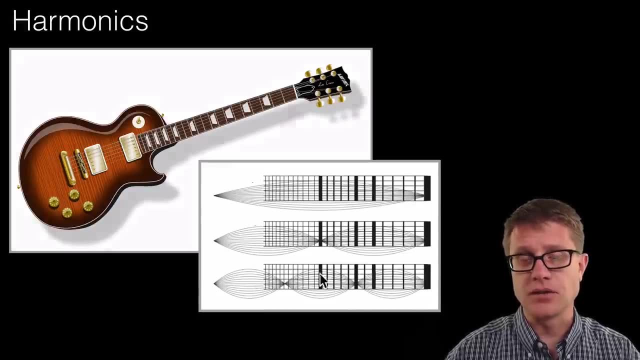 wave electrons is. we could think about fundamentals and harmonics. And so when you strum a guitar, this would be the first fundamental, This would be the second fundamental, The third fundamental. So, using that as a model, if we are looking at electrons, they are moving out from the center with different wavelengths. 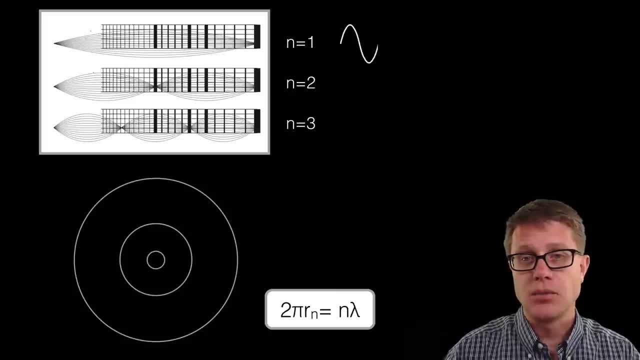 as well, And so let's start with the first inner electron. What is really going on is one wavelength is wrapping around the atom itself. What would that look like? if we look here at this first orbital, It is going to look like that. Now we know something about. 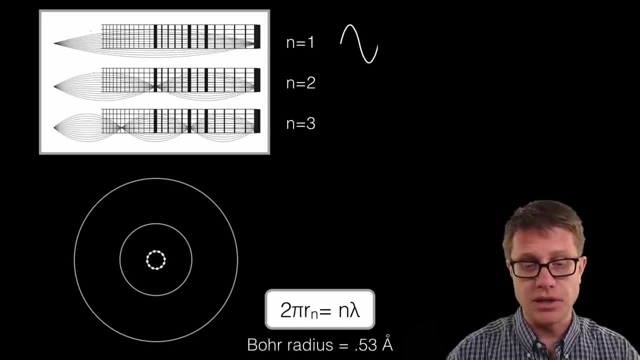 the momentum of the electron, We can calculate the de Broglie wavelength And if we plug it into this equation, this here is just is the de Broglie wavelength. And if we plug it into this equation, this here is just the original wavelength. So let's start with the. 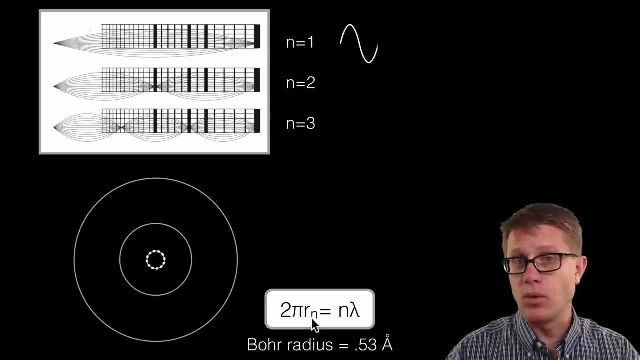 just the circumference of that circle, we can figure out what is the size of the atom, And it ends up matching up with the Bohr radius that we had measured before- 0.53 angstroms. Now what is the next level going to look like? Well, we have to have two wavelengths in there. 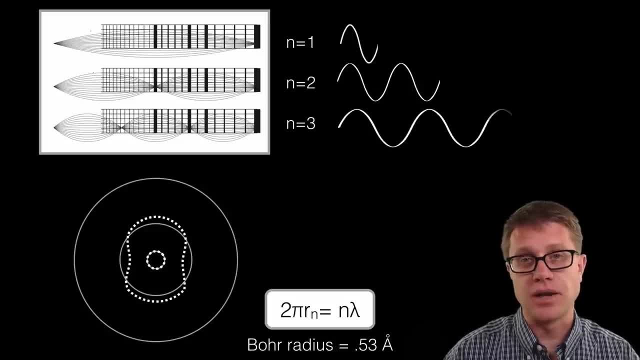 So what is that going to look like? It looks like that, And if we go to three wavelengths, we are going to have a different de Broglie wavelength, And so what are we going to get? It is going to wrap around like that, And so what is happening is the electrons are